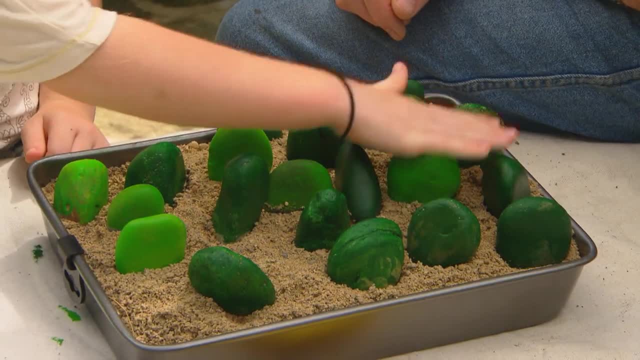 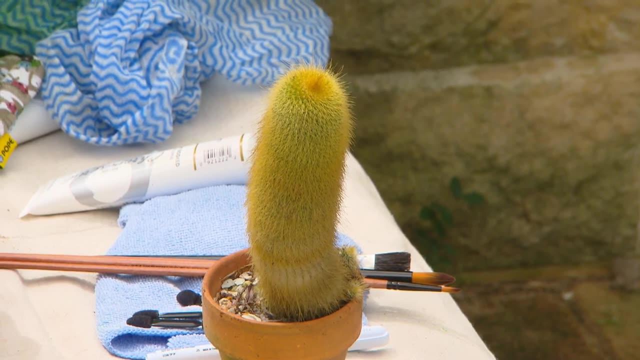 It is Next stage. are they dry? Yes, Good. Okay, Now we've got to paint the spines, just like this cactus here, But to do that we're going to need some white paint. Okay, grab your rock and paint your spines. 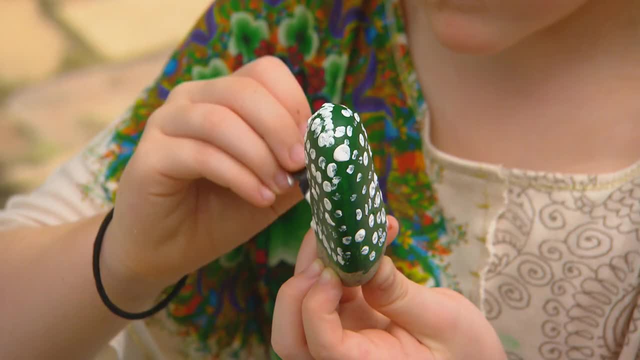 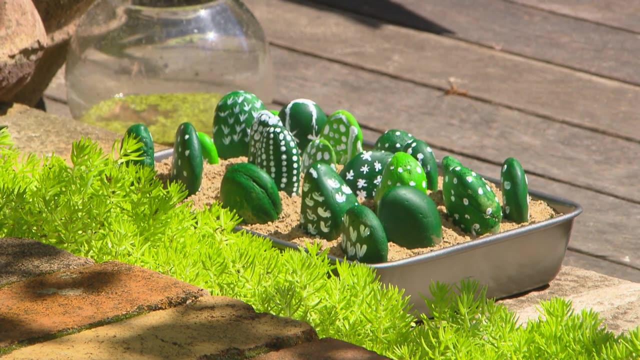 Now you've got to paint them on the other side. Okay, Plonk, Hey done. Okay, we'll put our cactus pebbles in the sun to dry. The next stage is to paint some pots, decorate them to put our cactus in. 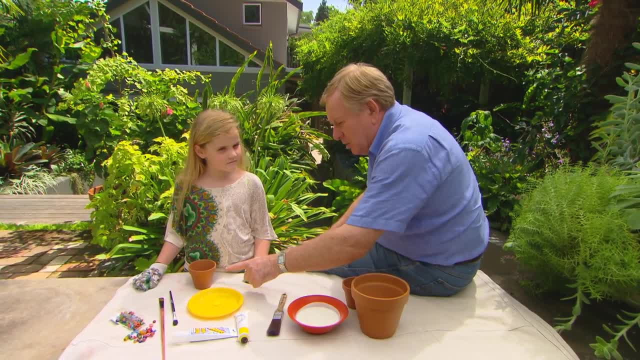 Now I think if you painted the bottom of that one with that beautiful golden yellow- and I'll paint these with yoghurt, Yoghurt, Why yoghurt? Oh, it gives you a really interesting finish. That is very good. 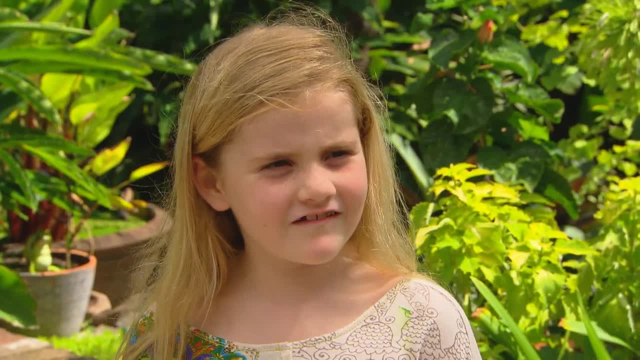 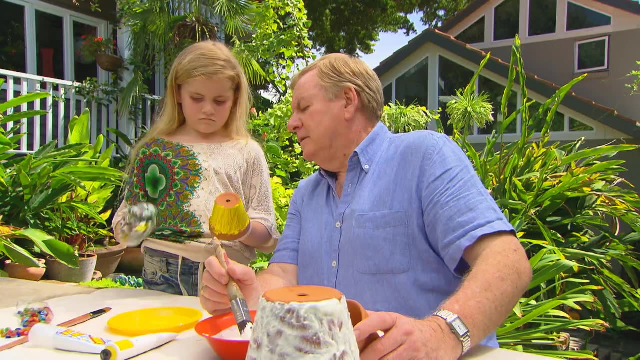 Artistique. Do you like my yoghurt? Want a lick? Now the next stage. if I put some glue on here, Do you think you can put some glue on here? No, No, No, No, No, No. 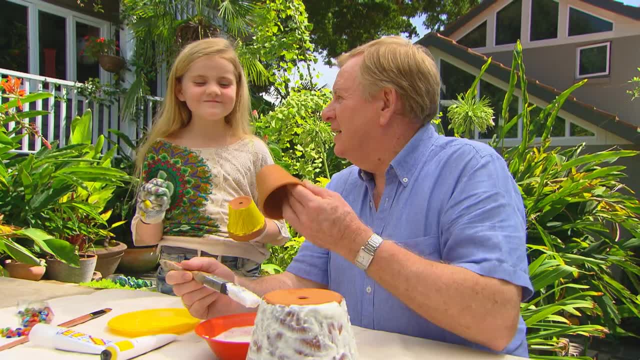 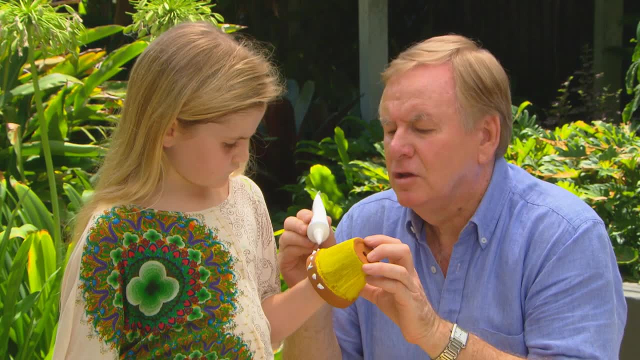 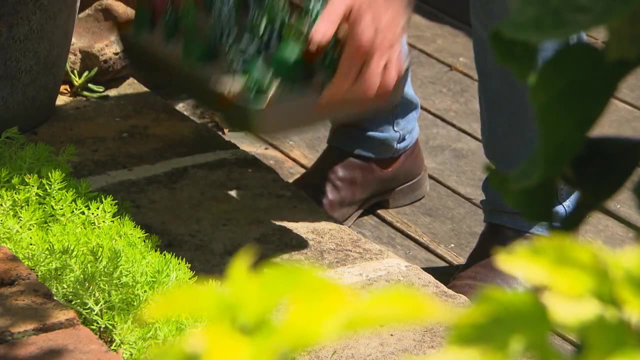 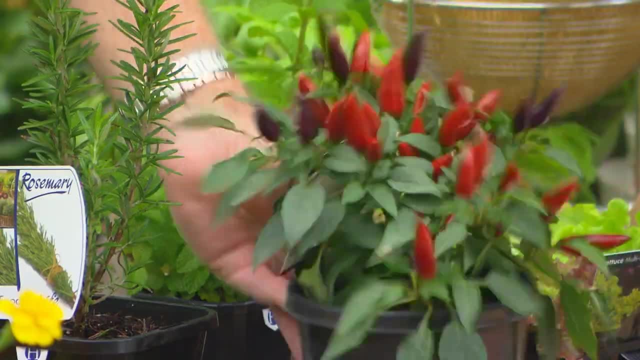 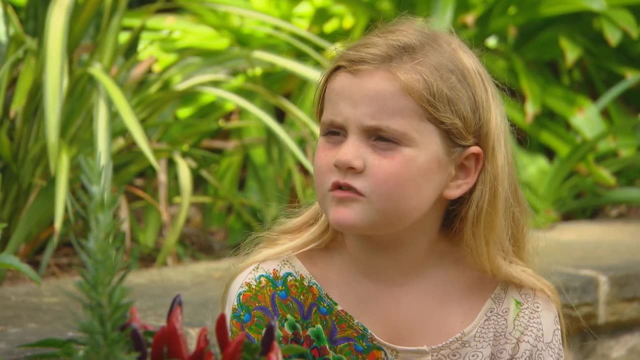 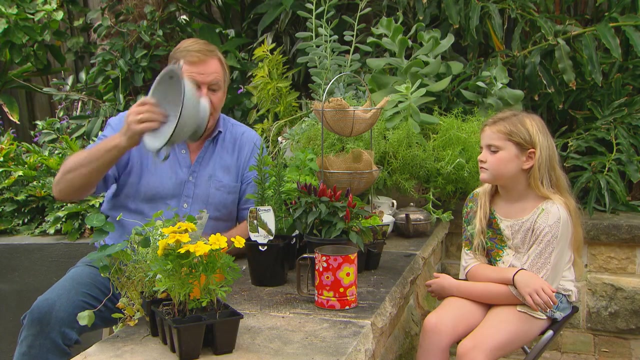 Remember, a little while back we bought these new bits and pieces in the kitchen. What happened to the old ones? Well, guess what? I kept them. There's a sieve, Oh, And a colander. You got a favourite herb. 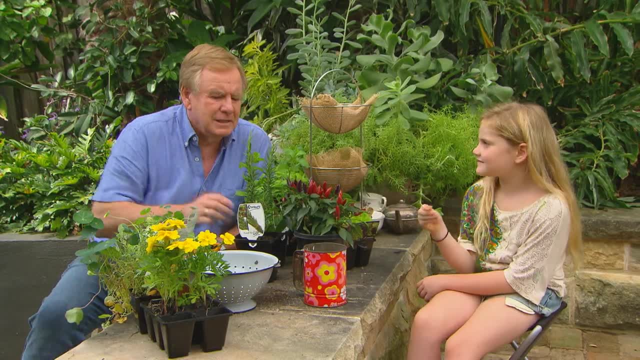 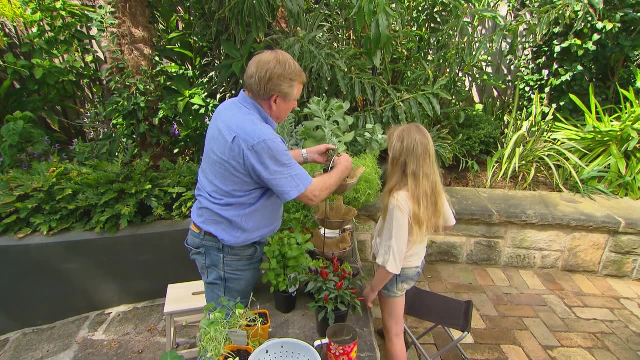 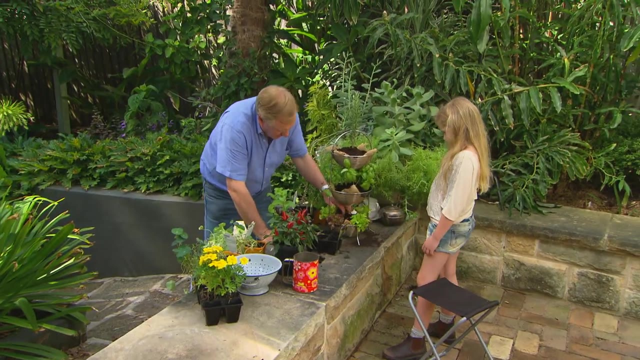 This one, The rosemary. You like it, Mm. Why's that? Because of the scent. Yeah, it does have a nice scent. I think we might plant it up the top there. Well, there you go, A great collection. 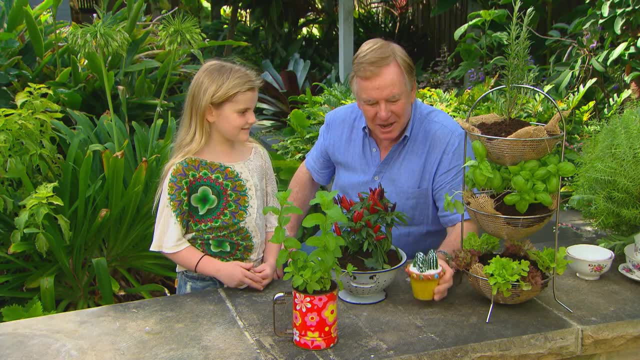 And have a look at these. Do you think Mummy is going to love these? Yeah, Why's that? Because I made them Well done.